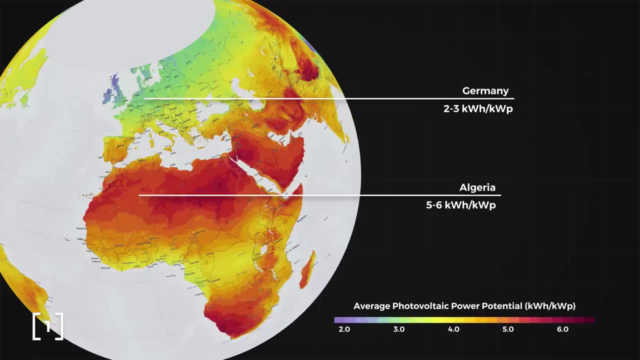 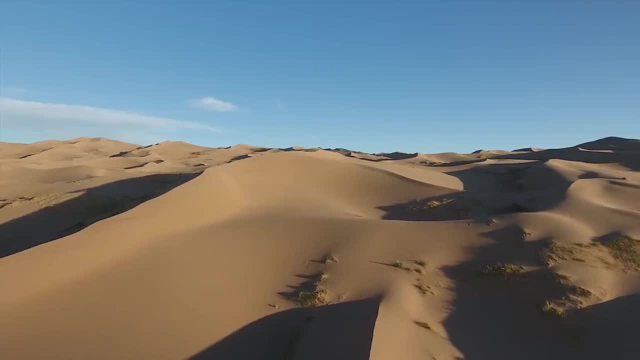 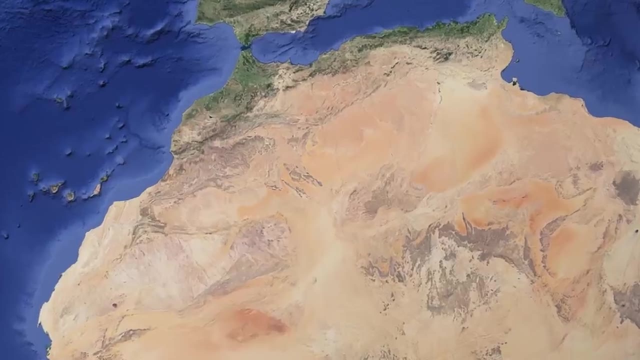 generating three times more electricity than the same panel placed in Germany. What was once a geographic disadvantage, the scorching sun of these desolate lands- could now provide an economic boom for these historically impoverished nations. A panel in a solar farm located here, one square metre in size, would, on average, generate: 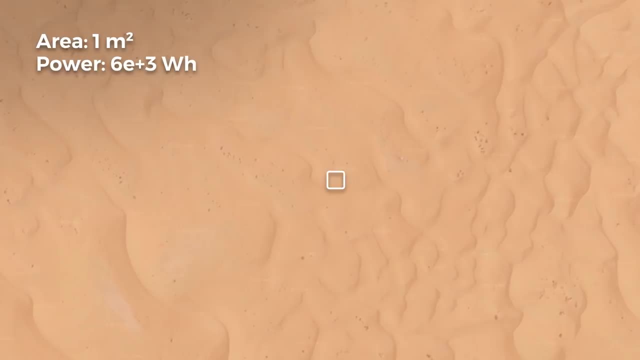 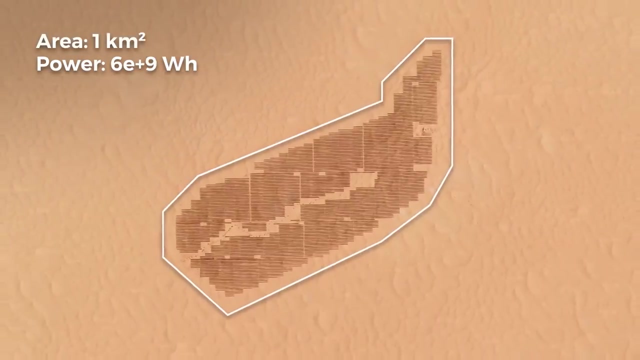 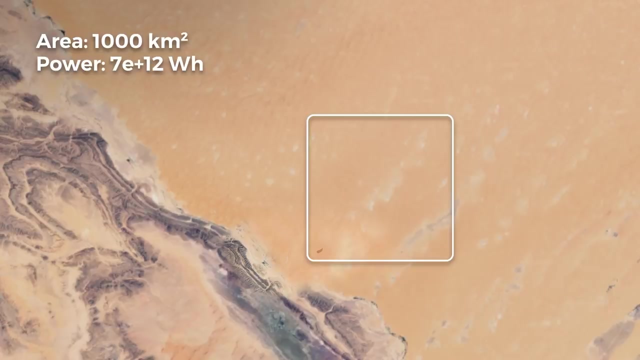 5 to 7 kilowatt hours of energy each day. Increase that to 1 square kilometre. we are generating 5 to 7 gigawatt hours of energy each day. Increase that to one second to 1000 square kilometres, and we are generating 5-7 terawatt hours of energy each day- enough. 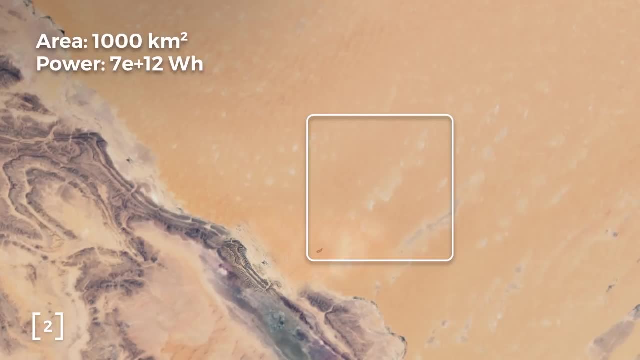 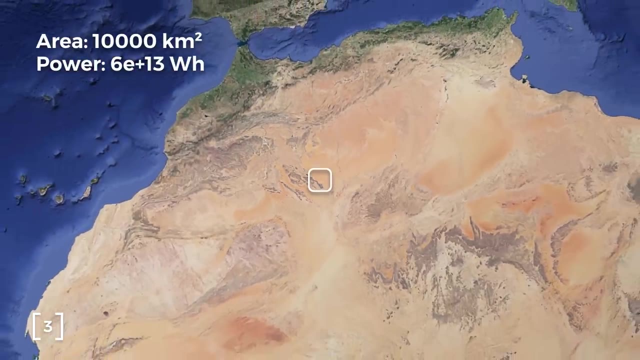 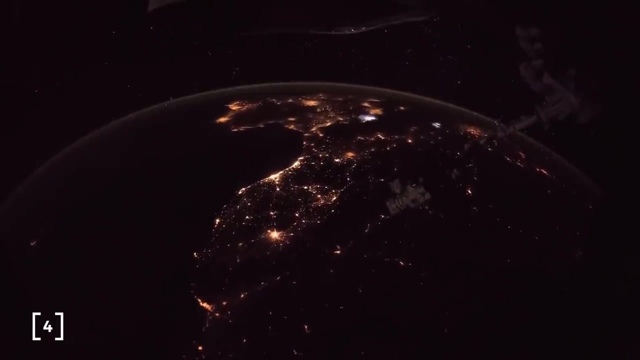 to satisfy nearly 100% of Europe's energy needs. Multiply that by 10, and we are generating 50-70 terawatt hours a day, enough to power the entire world. This is an impressive and often repeated statistic napkin calculations that draw a drastic new. 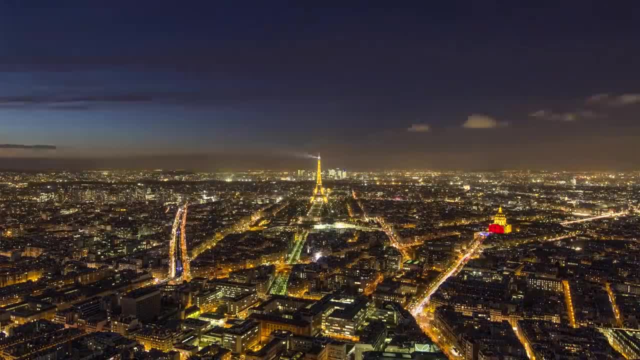 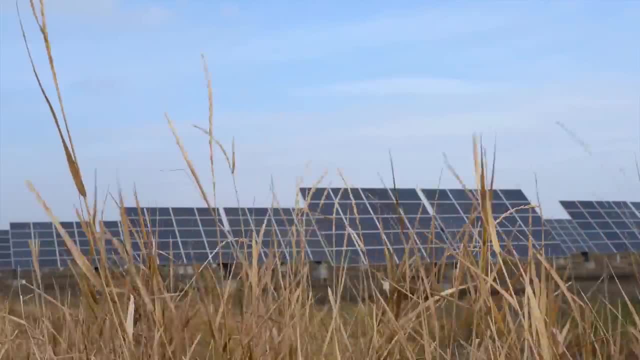 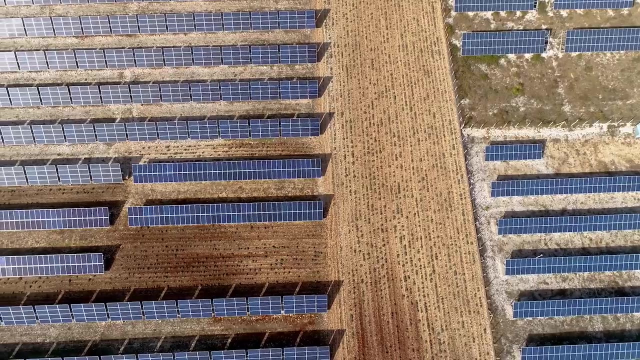 vision of the world, A solar powered utopia. Plans have even been drawn up to transform the simple mathematics into a reality, But reality has a way of interfering with futuristic pie in the sky calculations like this. Every plan to turn this dream into reality has failed. 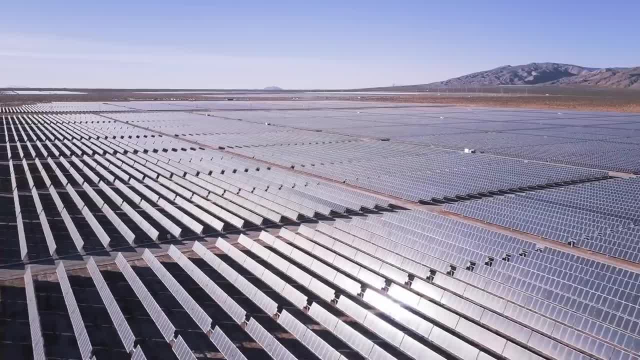 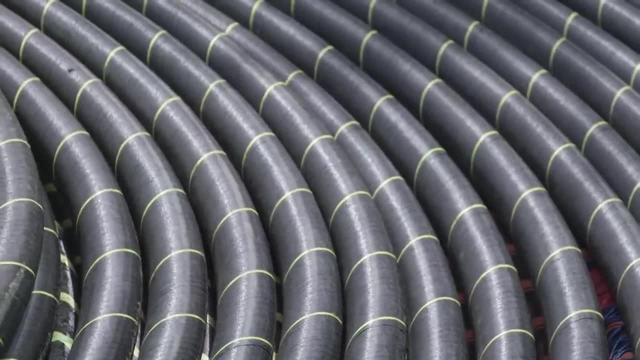 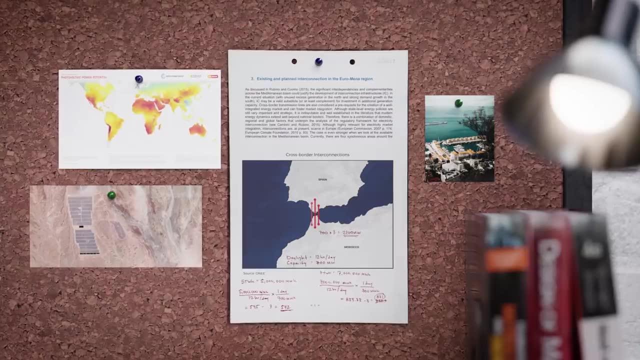 In this episode, we are going to learn why Transporting electricity out of these remote regions is the first challenge. Currently, there are only two interconnections connecting North Africa to Europe. Both are located between Morocco and Spain, Two 700 megawatt interconnections. 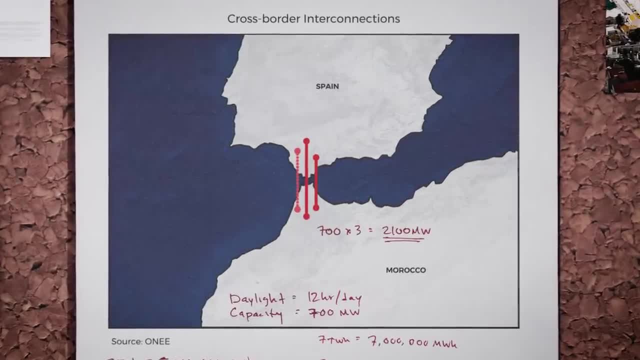 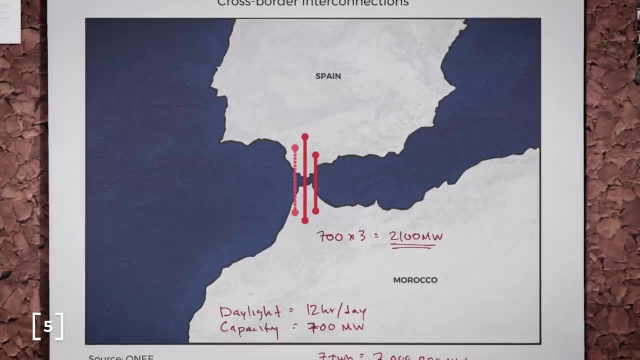 One completed in 1998, and the second completed in 2006,, with a third connection expected to be completed sometime before 2030, for a total of 2100 megawatts, If we wanted to transport enough electricity to power Europe. 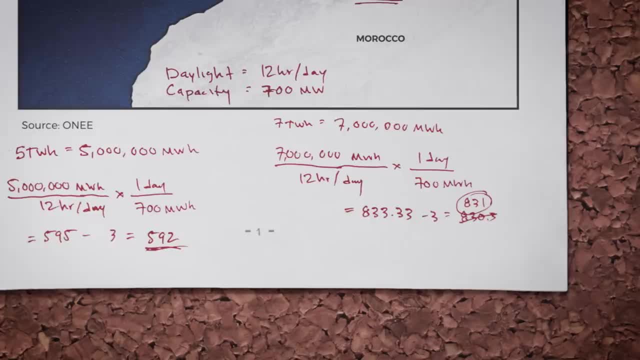 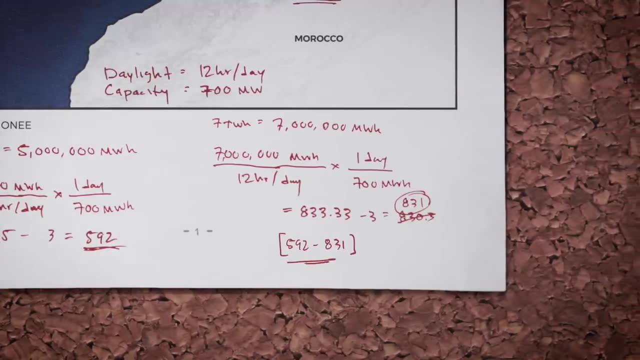 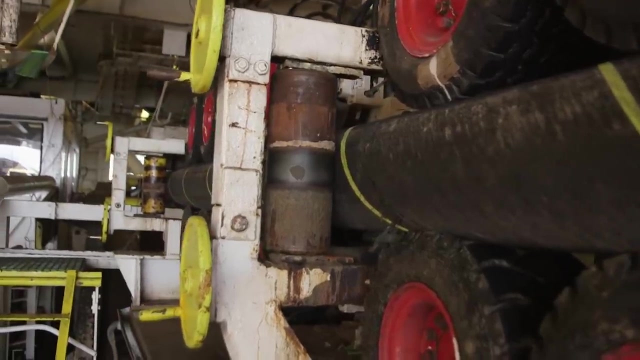 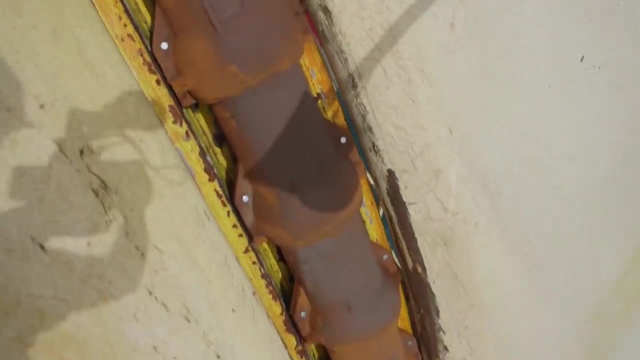 Ignoring transport losses and storage issues. We would need 592 to 831 more of these 700 megawatt interconnections. These aren't just simple cables that we lay between countries. They are incredibly complicated and expensive pieces of infrastructure. The third interconnection, joining Morocco and Spain's grids, is estimated to cost. 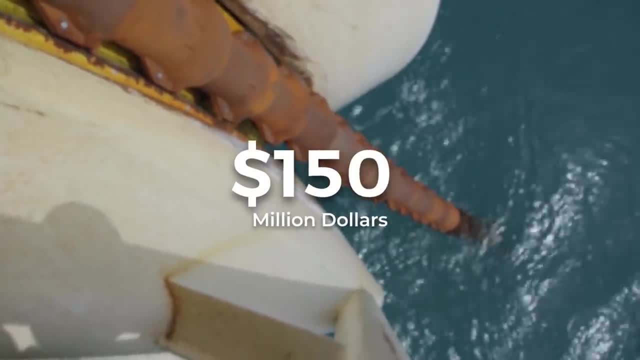 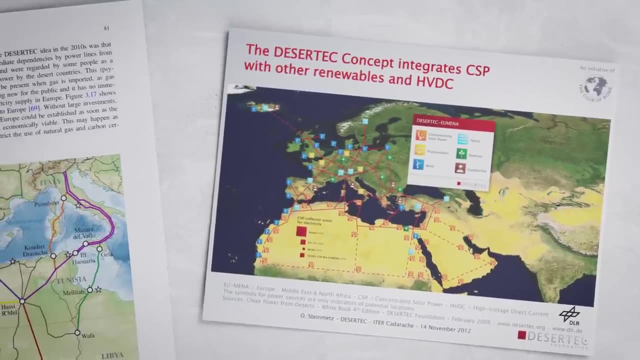 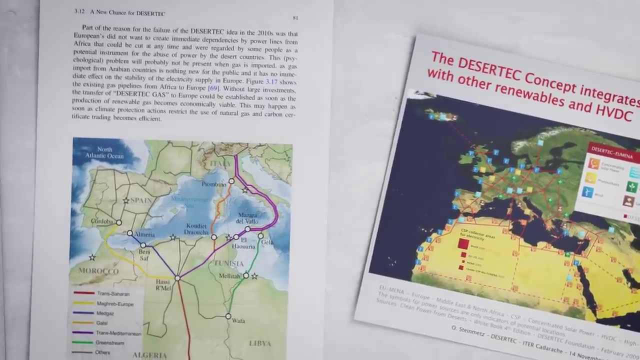 $150 million, An enormous investment That will see both countries footing half the bill. 592 more of these connections would cost, at an absolute minimum, $8.9 billion, And that number was found by simply multiplying 150 million by 592.. 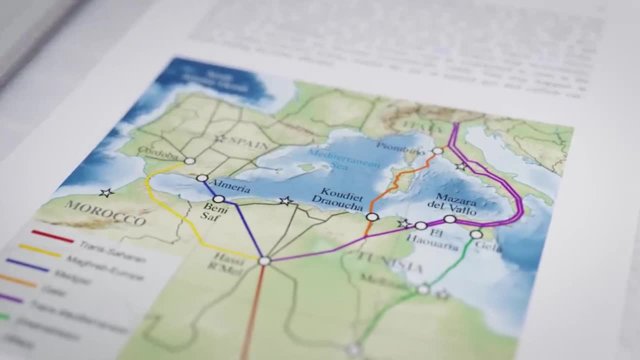 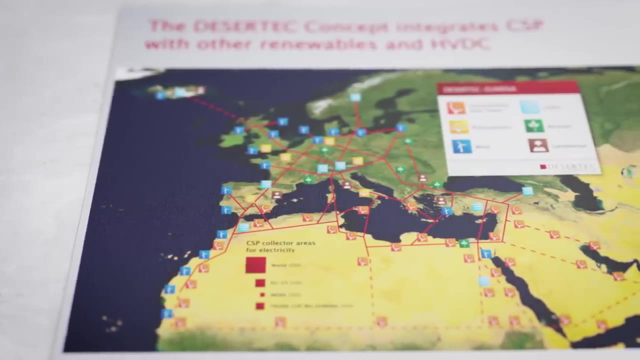 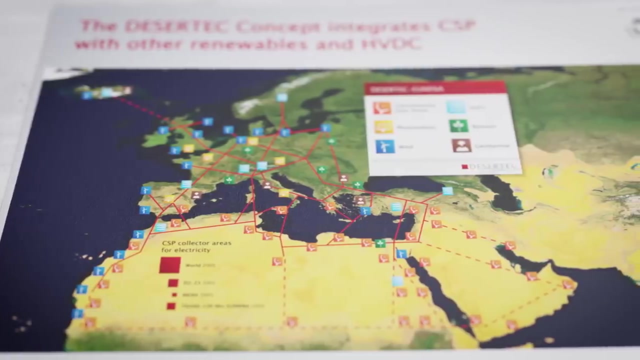 But these connections are the shortest route to Europe from North Africa. They are going to be the cheapest to build. To build a truly interconnected grid, we are going to need even longer interconnections Connecting Tunisia to Sicily, Algeria to Sardinia and onwards to Northern Italy, Libya to 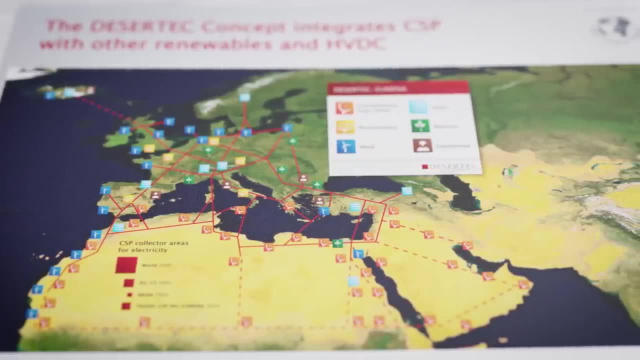 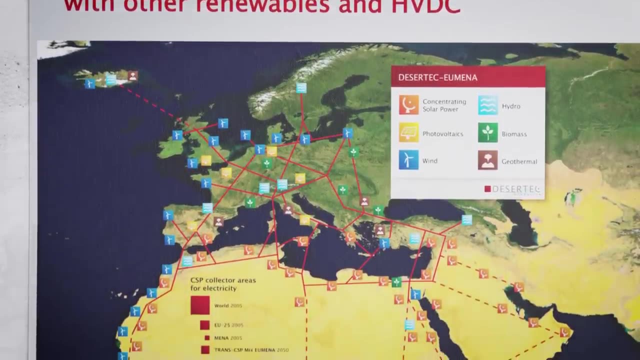 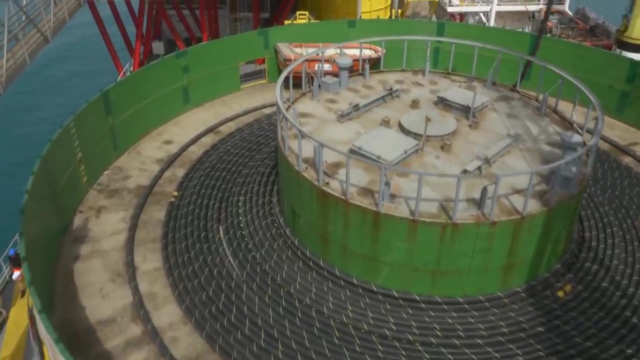 Crete and onwards to Greece and Turkey and to the rest of the Middle East network, All the while building enough internal interconnections in Europe to facilitate the passing of the solar parasol northwards while wind is traded south. This plan will take billions to complete. yet even with these issues, European leaders 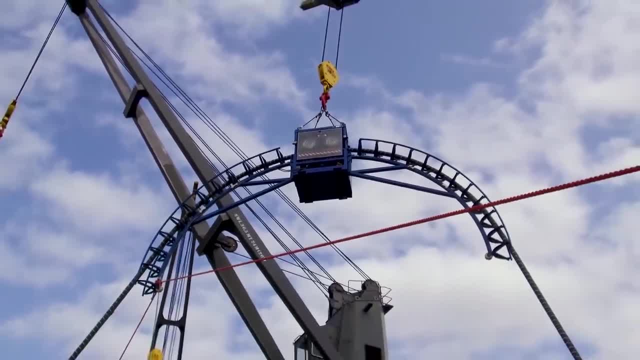 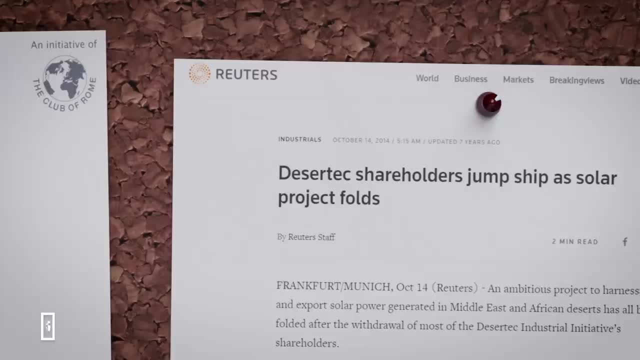 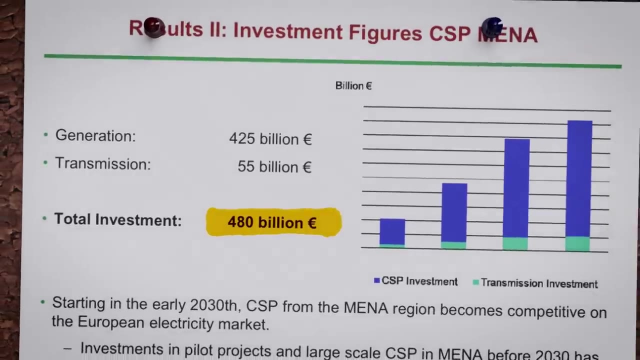 have drawn up plans to connect North Africa and the Middle East to Europe. They believe the cost can be recovered. Desertek is- or perhaps more appropriately was, a German led initiative centred around a half trillion dollar investment fund that would invest in generation and transmission. 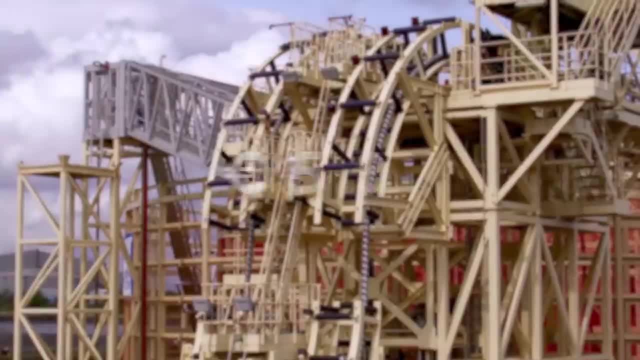 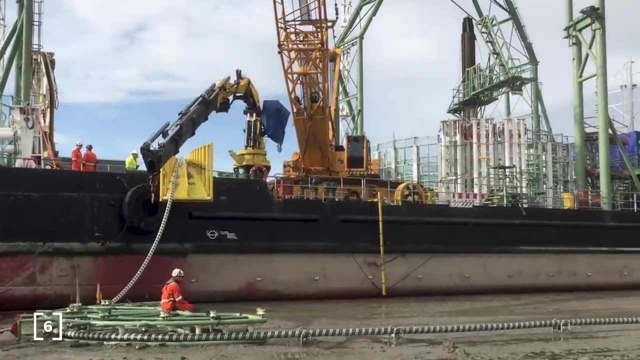 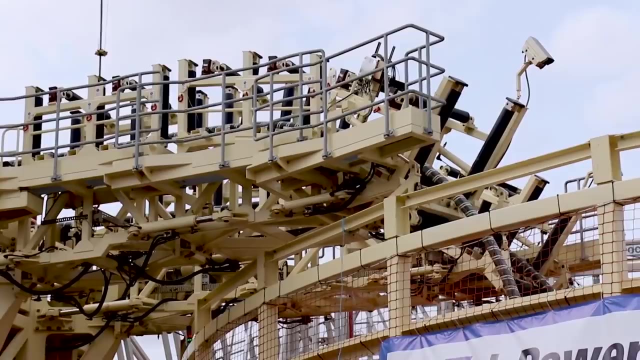 infrastructure across North Africa and the Middle East. $55 billion was allocated to increasing transmission capabilities across the Mediterranean. This investment would go into the development of a nuclear power plant. This investment would go into both high voltage alternating current transmission over shorter gaps, like those from Morocco to Spain, and high voltage direct current over longer distances. 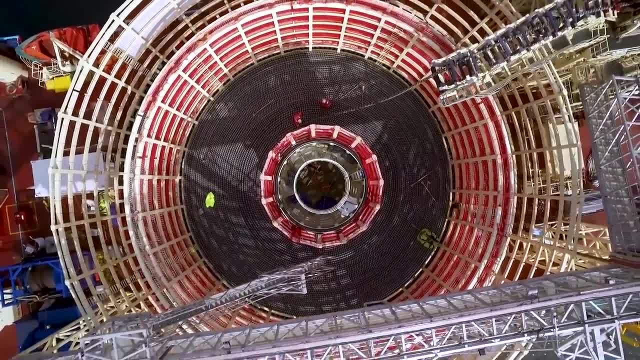 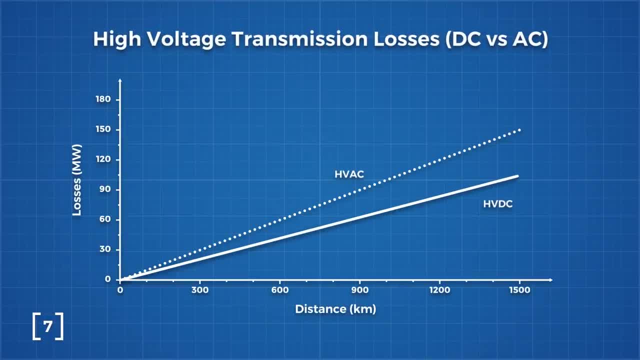 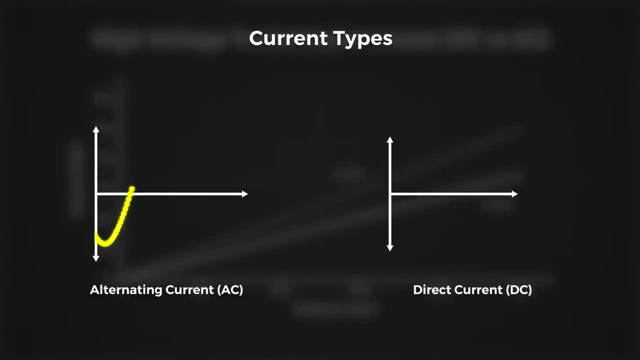 There is a critical distance where high voltage alternating current transmission does not make sense. If we plot transmission losses per kilometre for AC and DC transmission, it would look something like this, with DC losing less power per kilometre. However, In order to convert our regional AC grid power to DC for these long distance transmission, 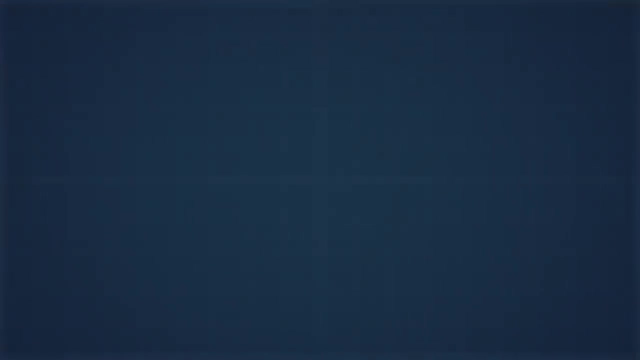 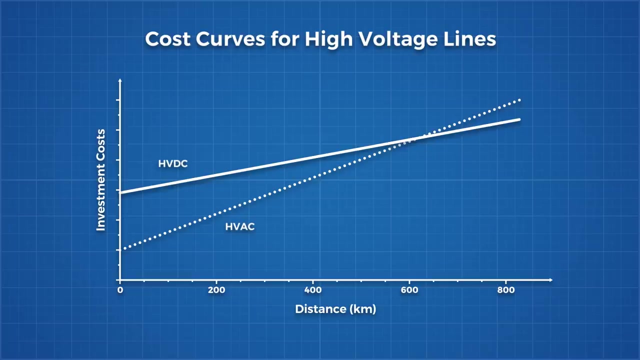 cables, we need expensive transformers and converters. If we instead plot cost versus distance counting in this infrastructure, it would look something like this, And we can see that the DC and AC lines cross each other around the 500-800 kilometre mark. 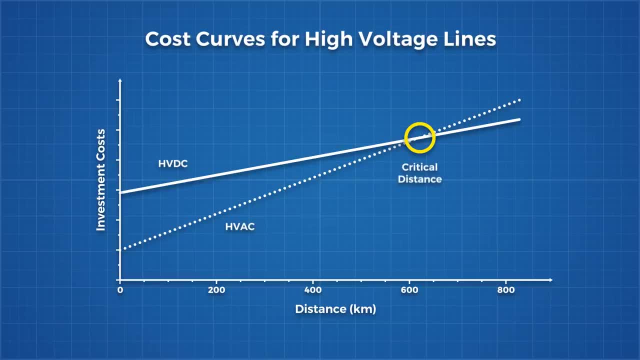 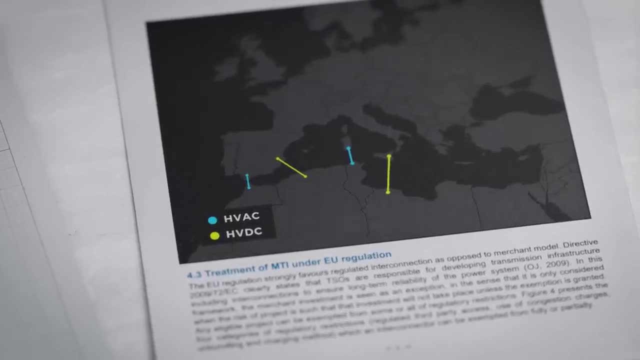 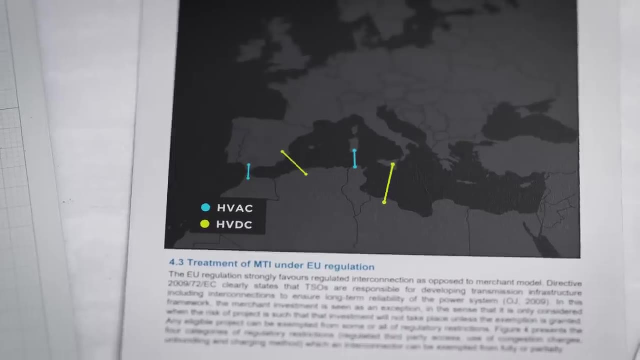 This is the break even point where DC becomes more cost effective. So The lines connecting Morocco directly to Spain, which spans only 28 kilometres, don't make sense for high voltage DC, while longer lines connecting Tunisia to Italy will likely be high voltage direct current lines. 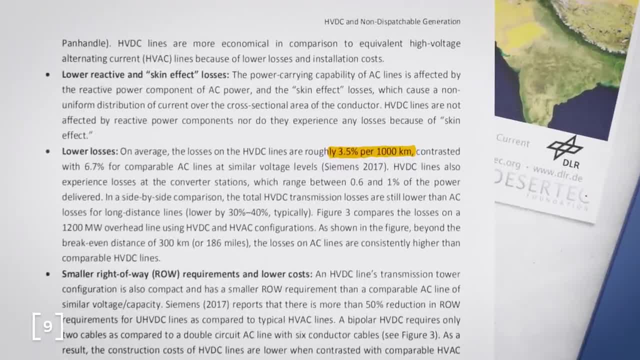 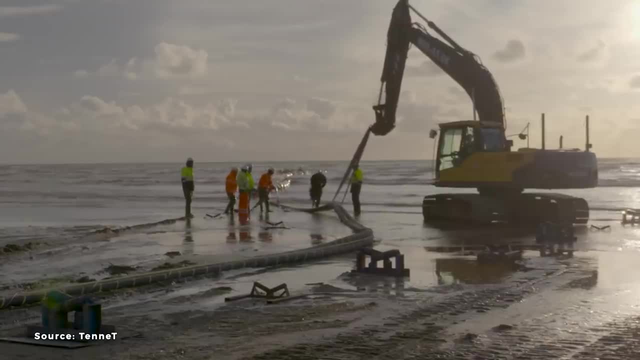 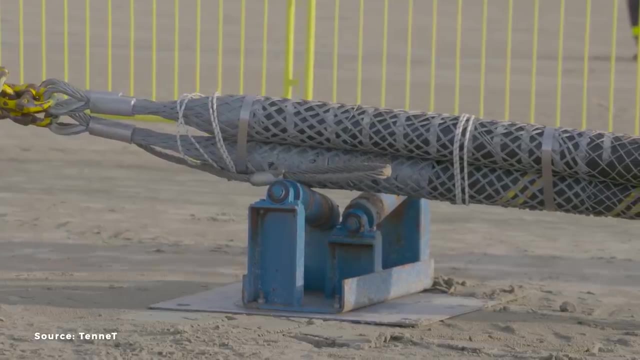 Transmission losses for high voltage direct current is about 3% per 1,000 kilometres, and Germany's capital is only 1,800 kilometres from Tunisia. Transmitting power with this much investment money is perfectly feasible. The technologies exist, so let's move into the generation. part of the DESERTEC plan. 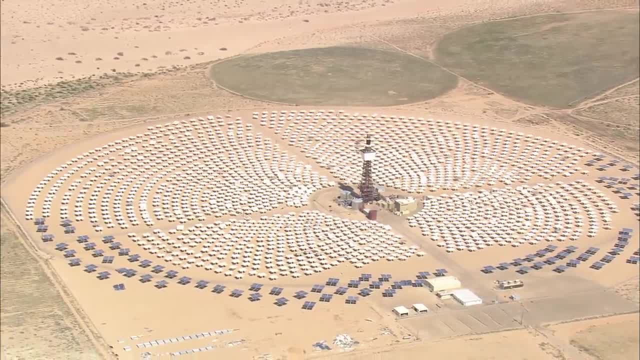 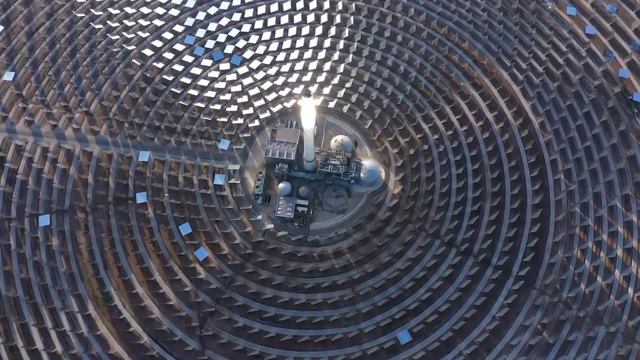 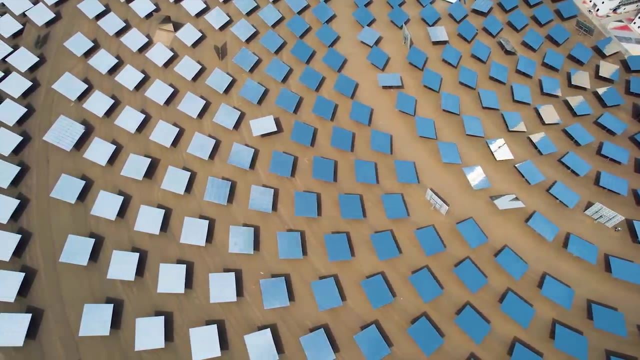 DESERTEC was formulated with concentrated solar power in mind, which works very differently to photovoltaic solar panels. Concentrated solar power facilities would be spread out along the borders of the Saharan and Arabian deserts. One such facility already exists in Morocco, and it's the largest concentrated solar 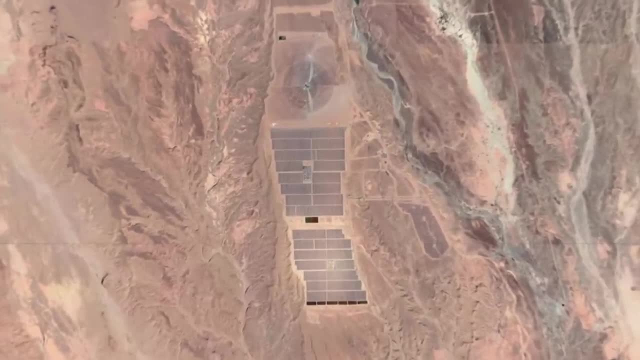 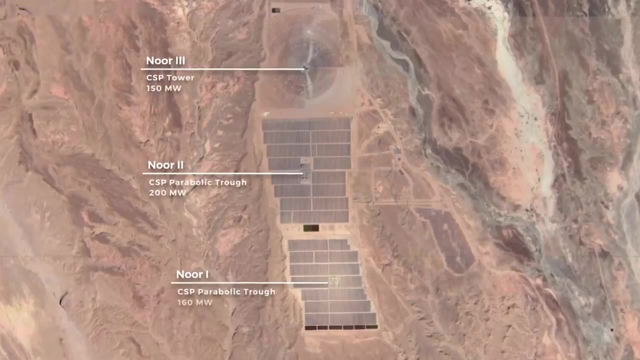 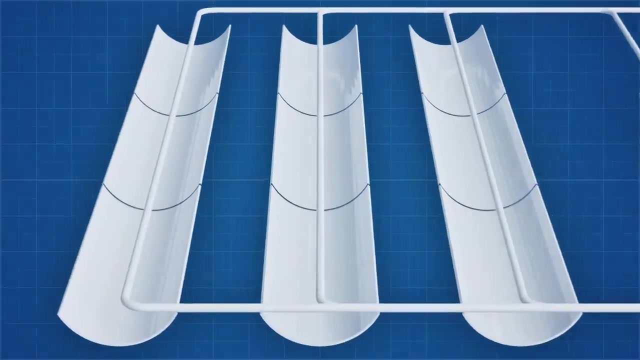 power plant in the world. It is massive, with three separate sections- NOR-1, NOR-2 and NOR-3,, each using slightly different variations of concentrated solar power, combining to provide 510 megawatts. NOR-1 and NOR-2 are both trough based systems that use parabolic mirrors with the tube. 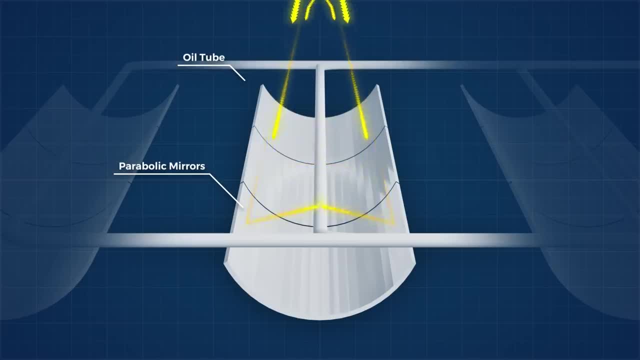 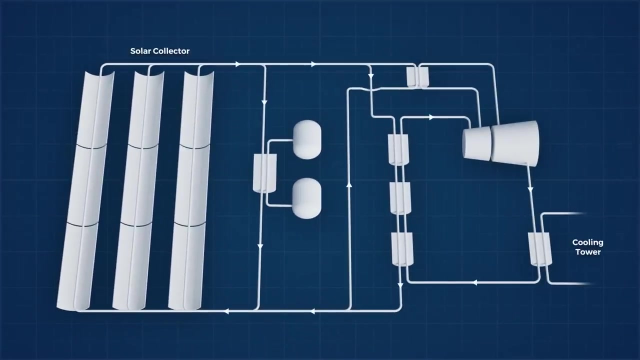 located in the mirror's focal point. The tube contains a synthetic oil which collects the heat from the 500,000 parabolic mirrors spread out over 308,000 square metres. This oil becomes extremely hot, as high as 400 degrees celsius, which allows it to boil. 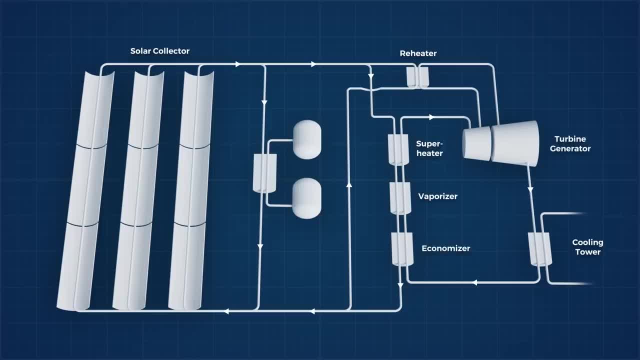 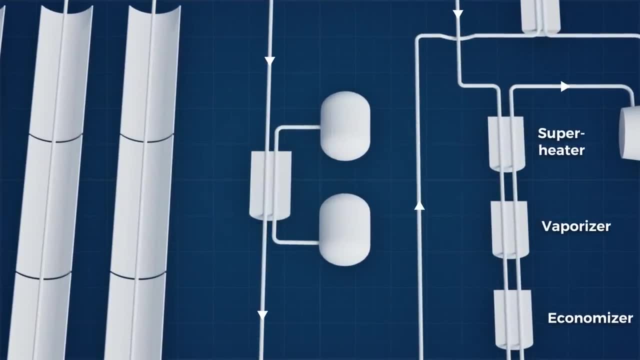 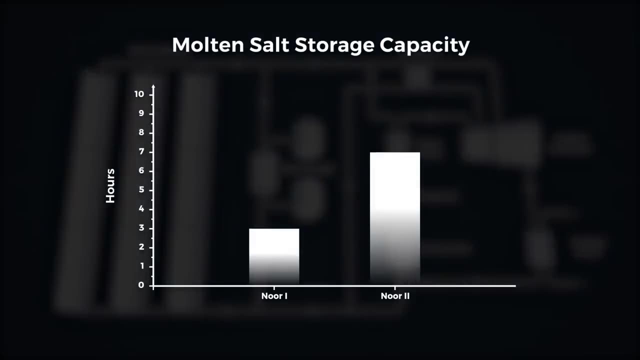 water in a heat exchanger to drive a steam turbine which provides electricity for the grid. The 400 degree oil is also hot enough to melt salt in a molten salt heat storage system. The molten salt heat storage system of NOR-1 can store enough heat to keep the plant operational. 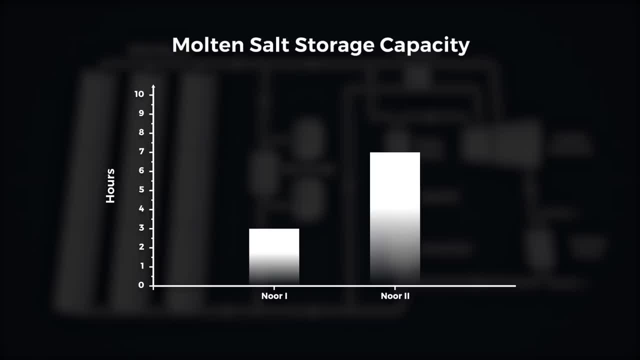 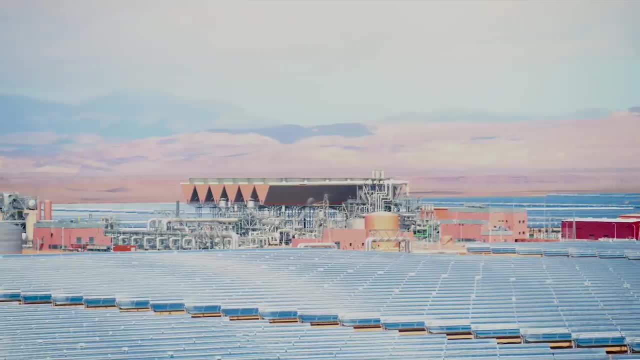 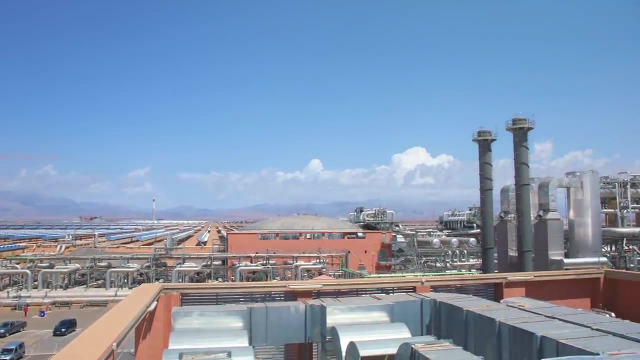 for 3 hours, While NOR-2 has enough energy for 7 hours. However, this salt solidifies at 110 degrees and if that happens, the plant won't work in the morning. So NOR-1 and NOR-2 need a fossil fuel burning system to keep all the working fluids of the 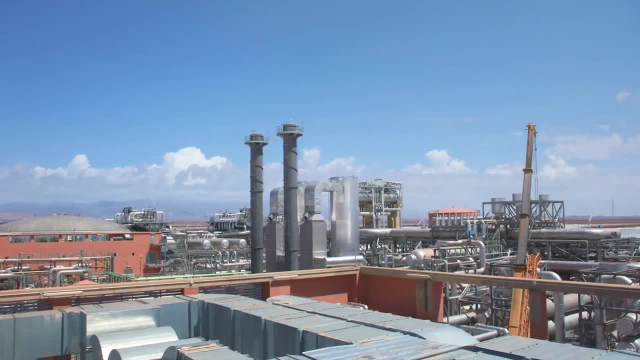 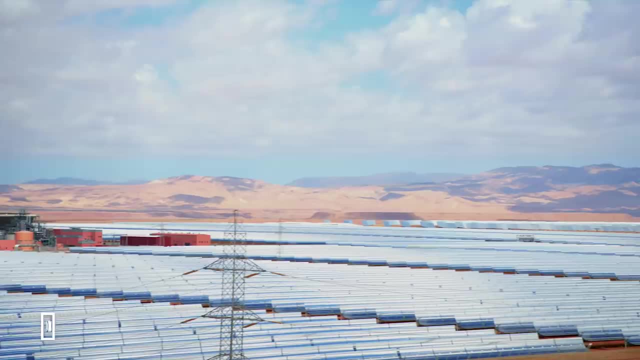 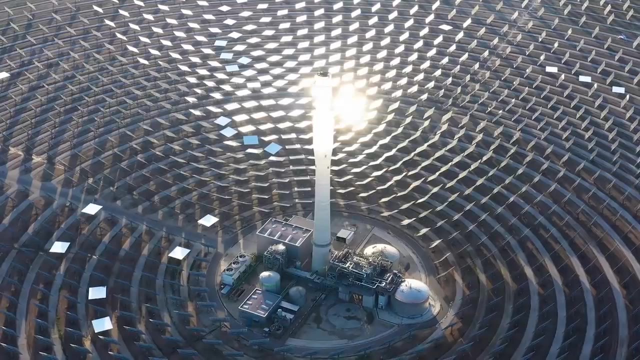 system at minimum operating temperatures overnight and to keep the oil system pumping. This fossil fuel burning system can also keep the plant operational as a reliable baseline energy source, removing the need for separate natural gas peaker plants. NOR-3 does not use these parabolic mirrors and instead uses a tower system. 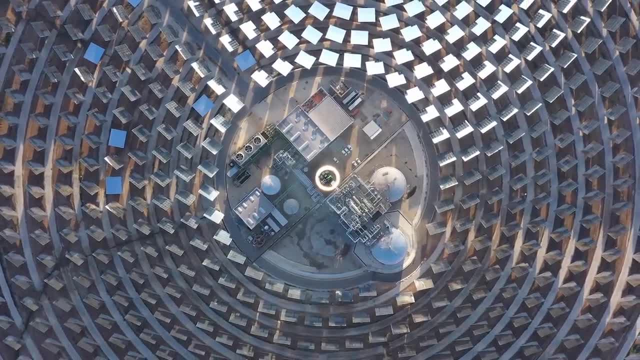 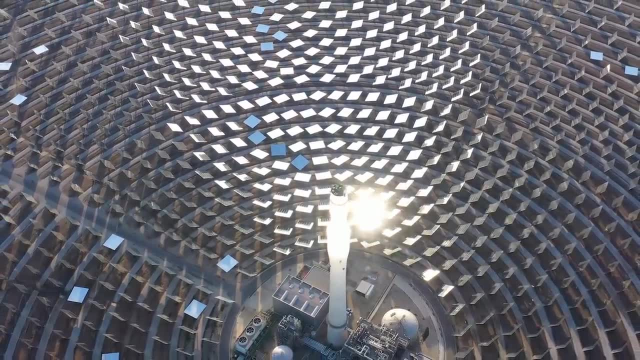 It's this striking circular facility. to the north It looks less like an industrial facility and more like a new age burning man art installation. This design allows NOR-3 to rid itself of the oil plumbing and pumps of NOR-1 and NOR-2,. 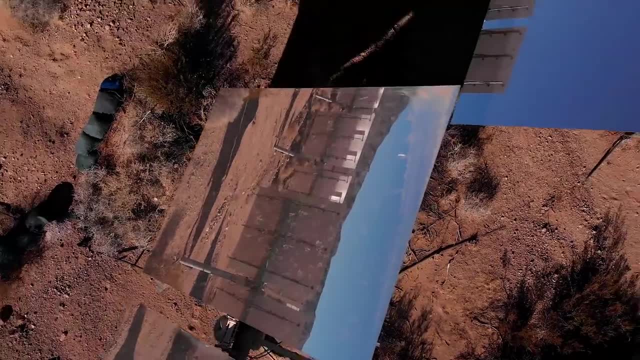 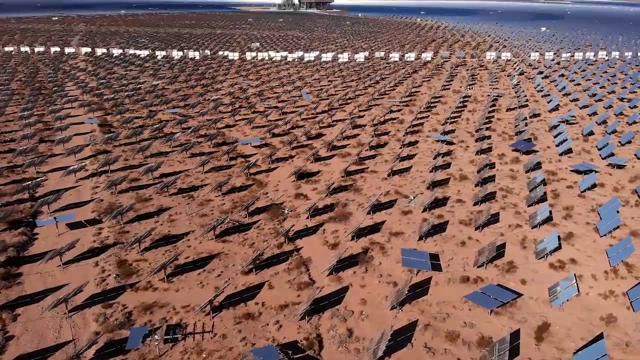 and instead it uses mirrors arranged in concentric circles around a central tower. The mirrors are then controlled to focus light on a single point on the tower which directly heats the molten salt, Which is the working fluid instead of the oil based system. 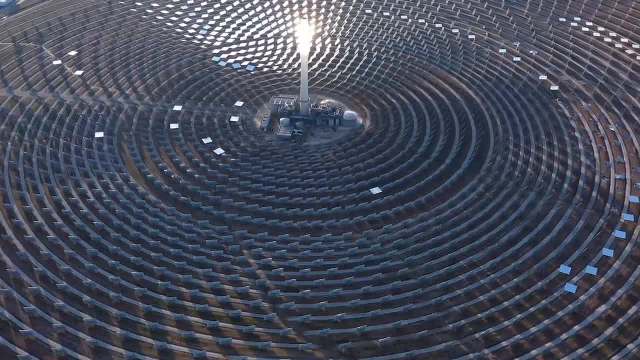 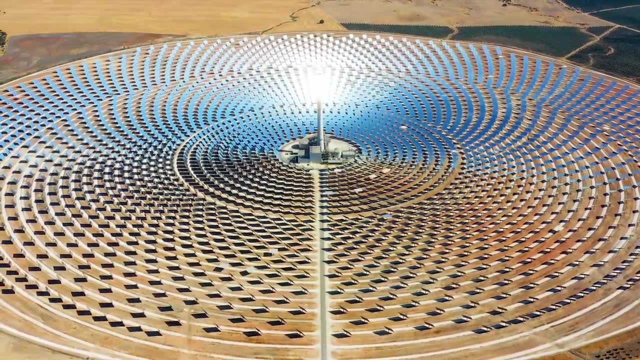 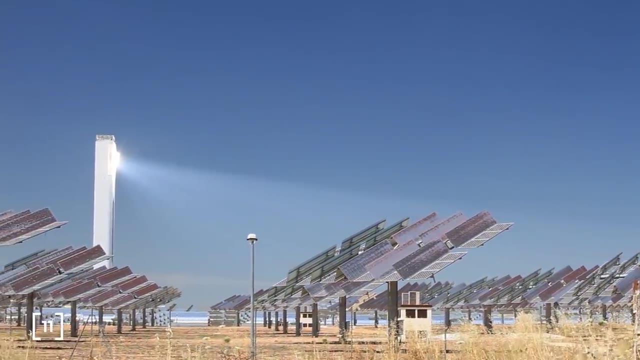 The solar concentration here is much higher and in turn, the temperatures attained are much higher, With the water being heated to 550 degrees. this allows the tower based system to use more efficient steam turbines, and using molten salt as the working fluid removes the need. 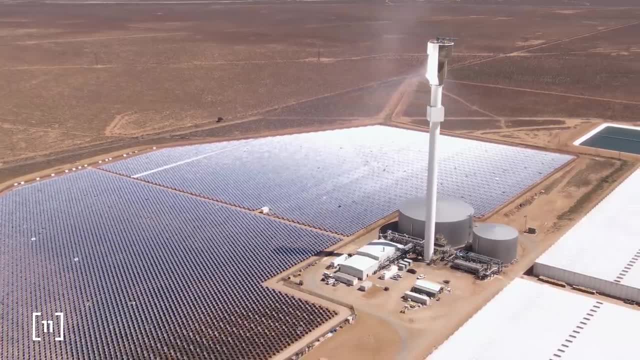 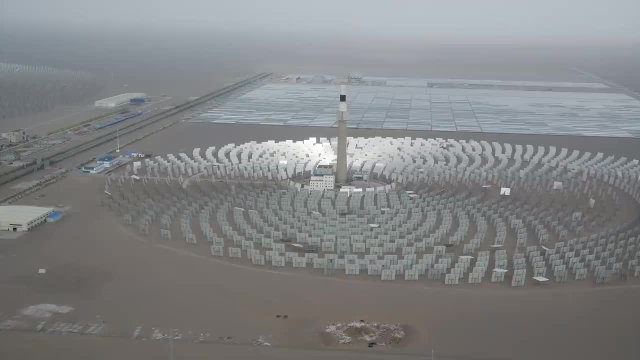 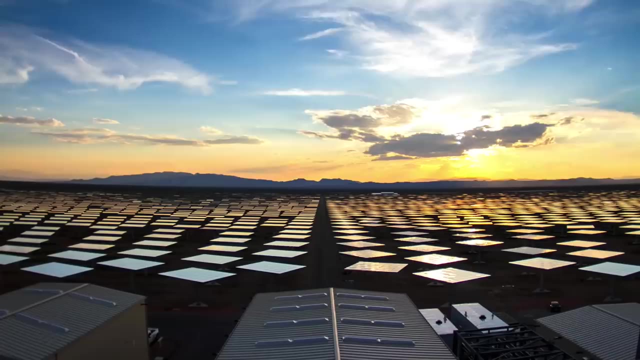 for an oil to molten salt heat exchanger in the heat storage system. NOR-3 is the world's only operating fuel burning system, The operating tower based concentrated solar power system with molten salt storage After 2019's shutdown of Nevada's Crescent Dunes plant. 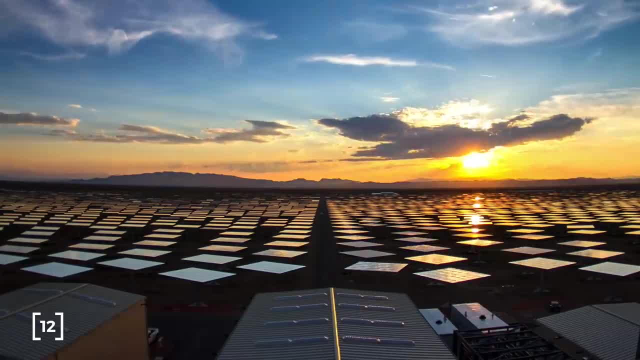 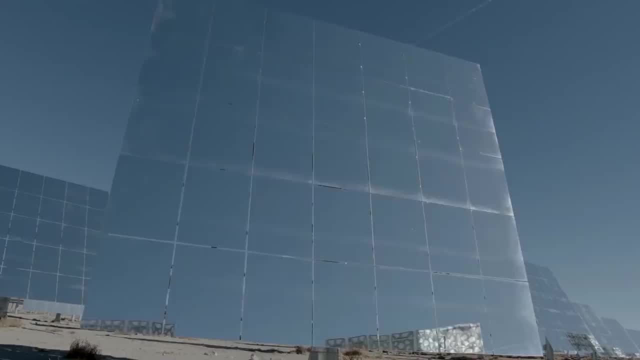 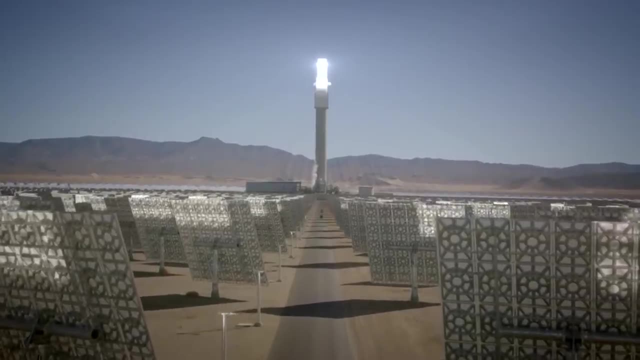 The Crescent Dunes plant ceased operation in 2019 after only 4 years of operation. NV Energy broke its purchasing contract with the plant after it failed to meet performance requirements, Being marred by maintenance issues, including an 8 month shutdown due to a leak in the molten. 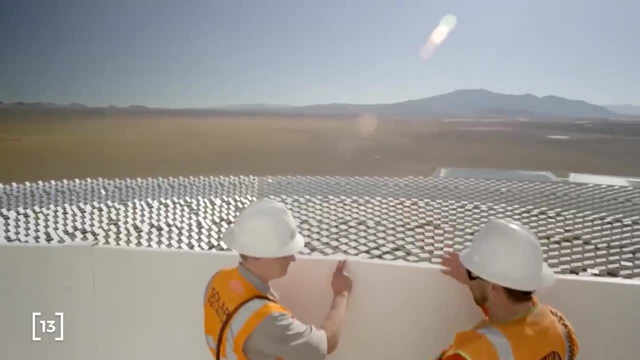 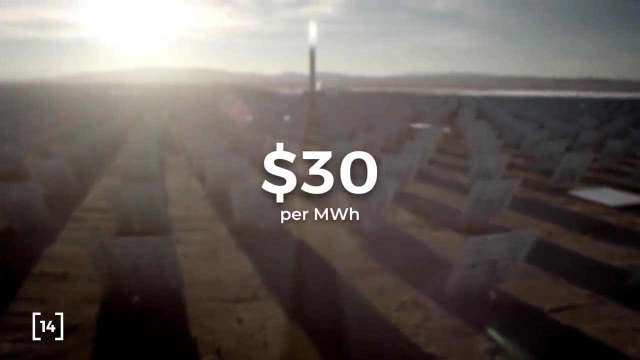 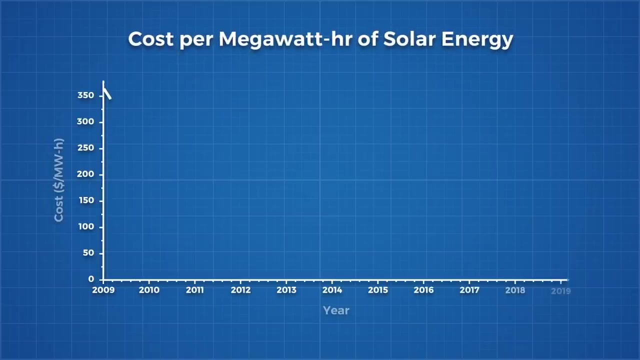 salt tank. Even when fully operational, the plant's electricity cost $135 per megawatt hour, while a nearby photovoltaic plant was managing $30 per megawatt hour. And here lies the crux of the issue. Concentrated solar power costs per megawatt was extremely competitive with photovoltaics. 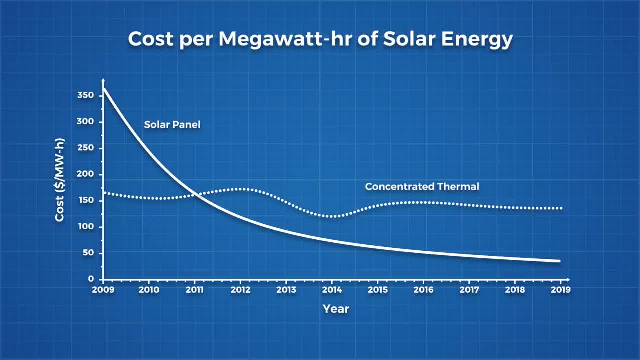 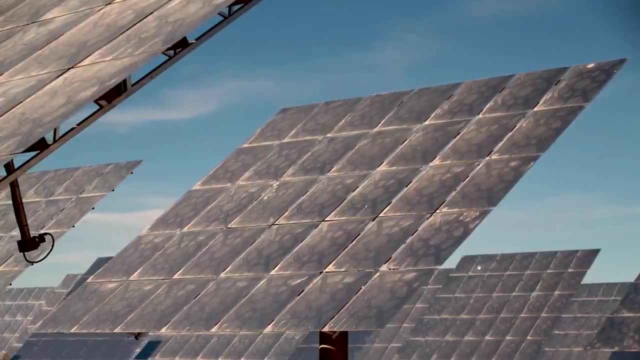 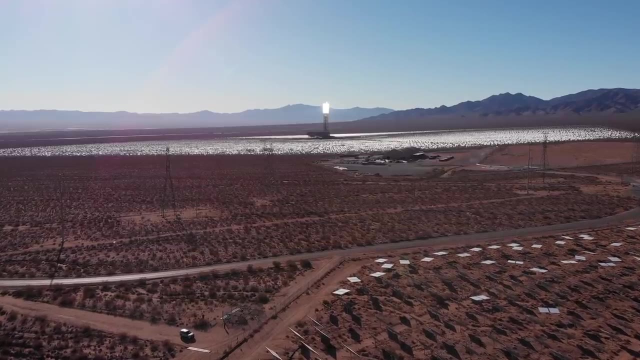 in 2009.. But in the last decade, photovoltaics have become obscenely cheap. Concentrated solar power simply cannot compete, And the same can be seen for NOR-1,, 2 and 3.. However, they are currently being measured on a metric called levelised cost of electricity. Which is an average of the cost to generate electricity over the entire life of the plant. But this does not factor in the cost of storage for photovoltaics, which is often just an inherent benefit of concentrated solar thermal power. So, Going forward, the industry should be using a combined cost of storage and cost of electricity. 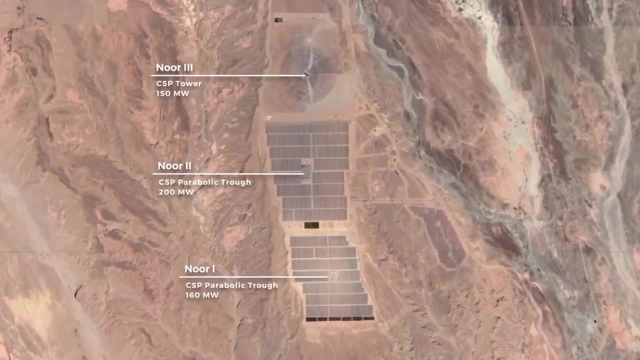 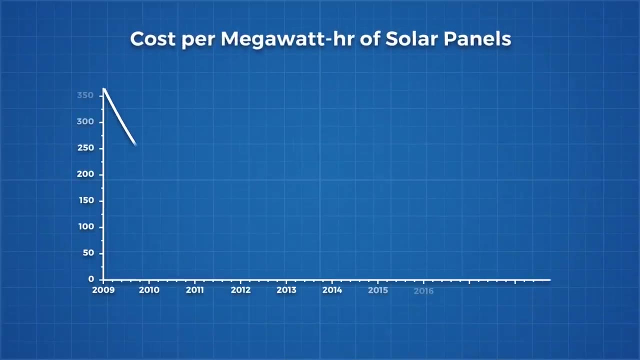 metric. Yet the most recent addition to this solar farm is NOR-4,, a solar panel farm contributing 73 megawatts. With the rise of cheap solar panels, DESERTEC, contrary to what you might expect, was doomed for failure. Concentrated solar thermal power by nature needs a lot of land. The plant has a minimum viable operating temperature And to achieve that we need enough mirrors to reflect that light. Solar panels do not have this problem. Solar panels can be fitted on top of homes, over car parks or even in farmer's fields. to help shade plants that need shade. We don't need massive plots of land to make them work, And because they are so cheap, it's perfectly feasible to build smaller solar farms in Germany and avoid those transmission losses And not incur the massive financial risk. And because they are so cheap, it's perfectly feasible to build smaller solar farms in Germany or avoid those transmission losses. And because they are so cheap, it's perfectly feasible to build smaller solar farms in Germany and avoid those transmission losses. And because they are so cheap, it's perfectly feasible to build smaller solar farms in Germany. 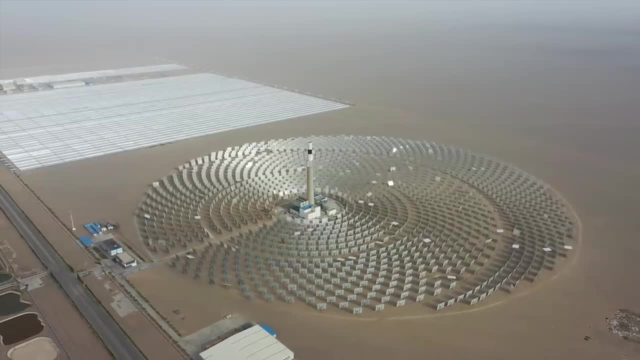 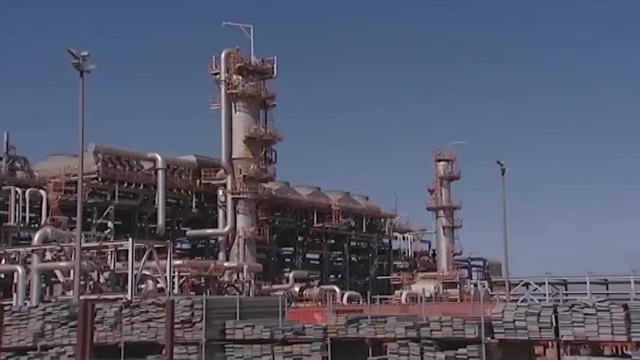 and avoid those transmission losses As a big part of the financial risk of investing billions into a country that is not your own. That's particularly important because a lot of investors are very hesitant to put money into these often volatile countries. We need to look no further than the 2013 attack on a BP natural gas plant in Algeria to see. 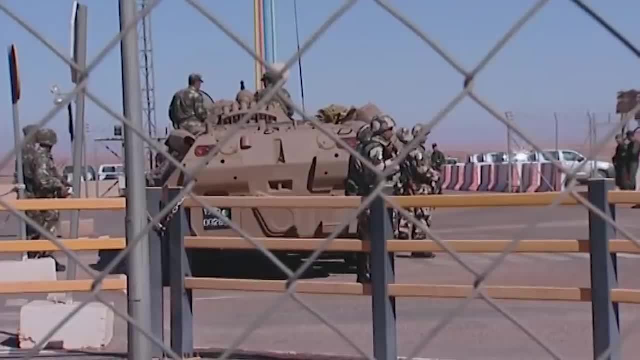 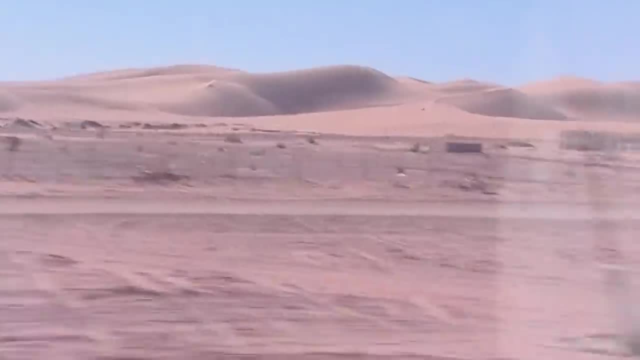 why this would be considered a risky investment in many parts of north Africa. It's a vital economic resource for Algeria, yet it sits on the top of the list of all thoughts, isolated in the midst of a vast desert that's a transit route for Al-Qaeda in North Africa. 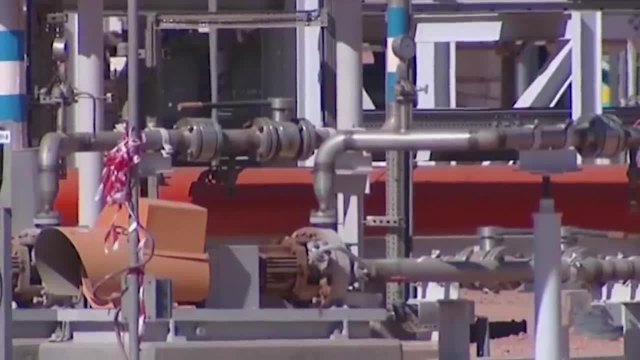 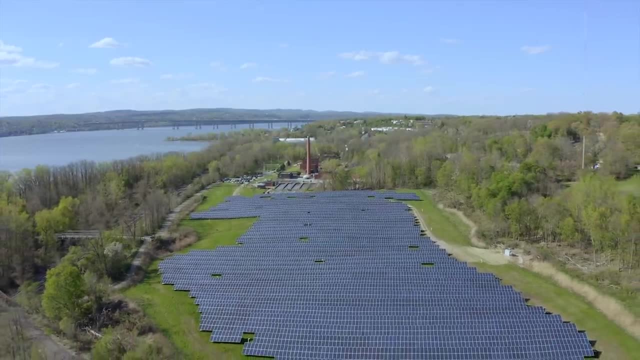 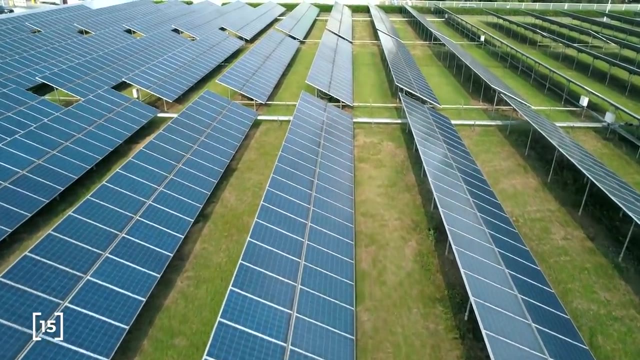 No wonder it was so difficult to defend and such a tempting target for the militants". This is all exactly why Germany is instead investing in its own domestic photovoltaic generation and in 2020, solar power accounted for 10% of Germany's power generation. 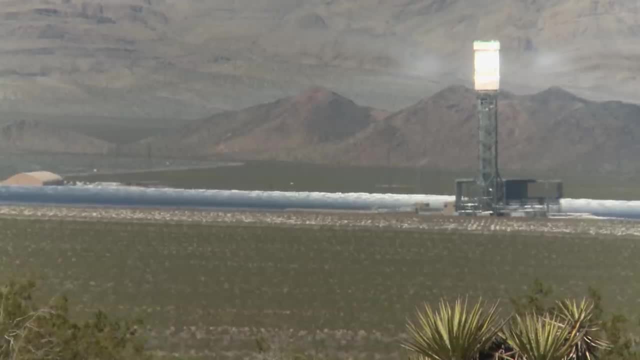 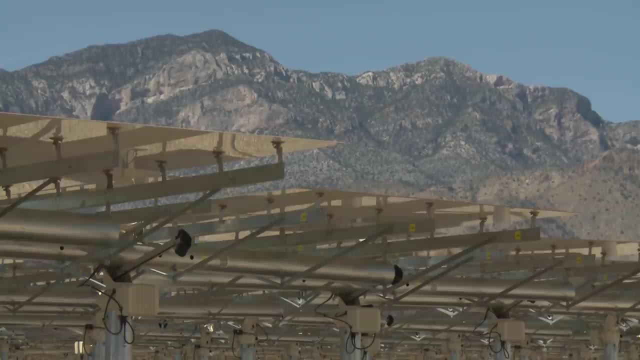 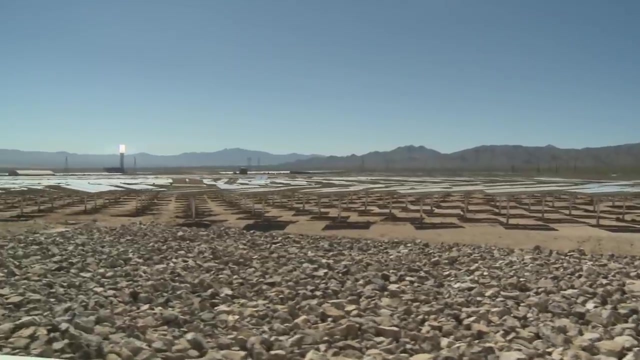 This idea of European countries drawing natural resources from Africa to benefit their own economy has some undeniable, problematic historic parallels. Any foreign investment like this is going to come with some guarantees of supply for Europe, Beyond the difficulties of organising cross-border cooperation like this. that's not going. 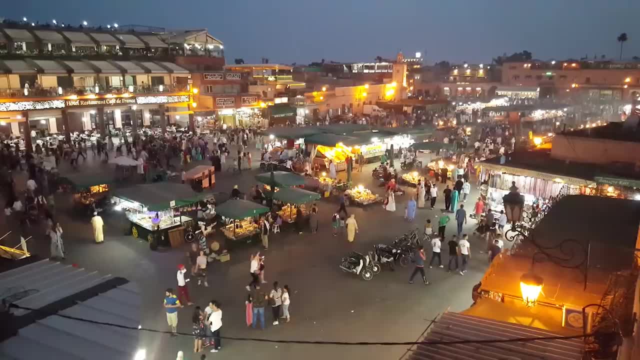 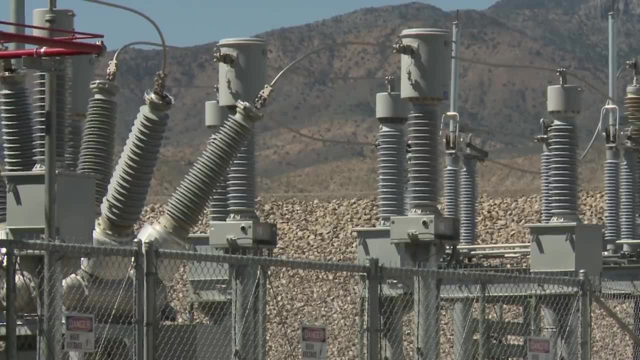 to go down. well, when the country hosting these plants needs that power for their own grid, To power their economy or simply stabilise their own grid for current needs. It becomes even more problematic When you consider the amount of water these facilities need for cooling for the steam. 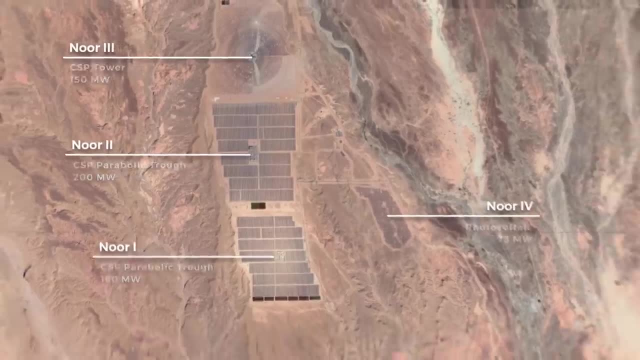 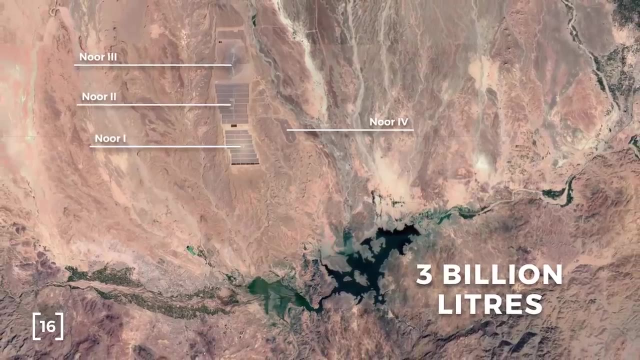 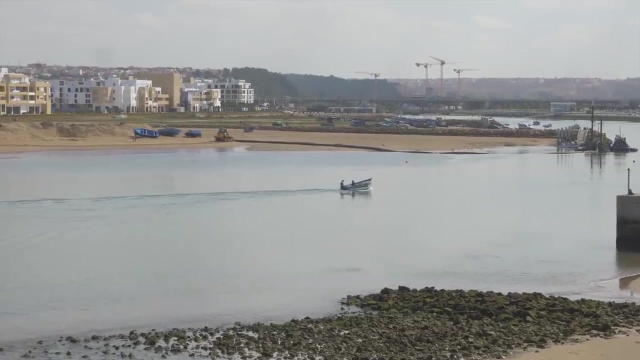 turbine and to keep the mirrors clean. This facility in Morocco uses 2.5 to 3 billion litres of water every year, taking water from a dam 12 kilometres away. Morocco is already susceptible to droughts, so scaling these water demands up just to. 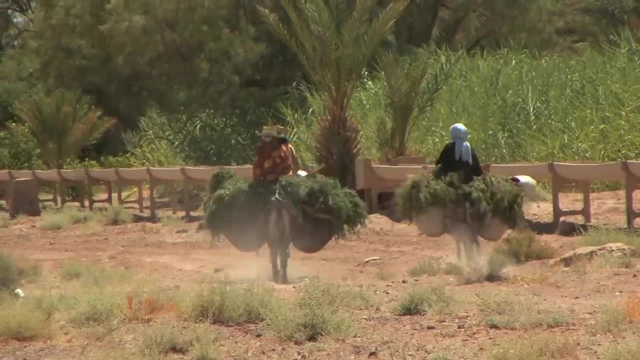 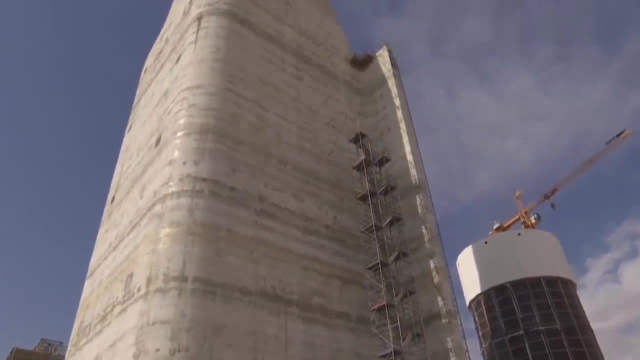 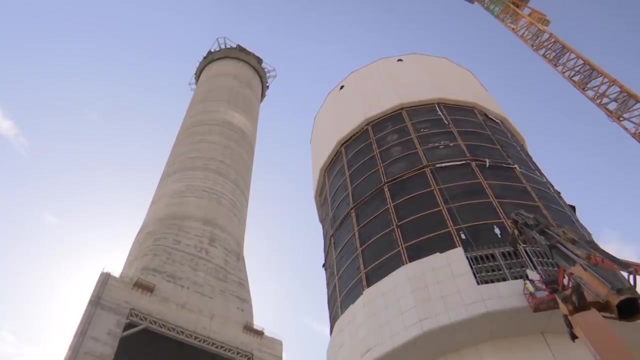 feed Europe's power needs, while taking water away from the farms that feed Moroccan citizens is even more problematic. So what's next? To truly scale this power generation, some technological improvement that reduces the consumption of water would be needed, Or just pair the facilities with desalination plants and use the extra water, if any, to 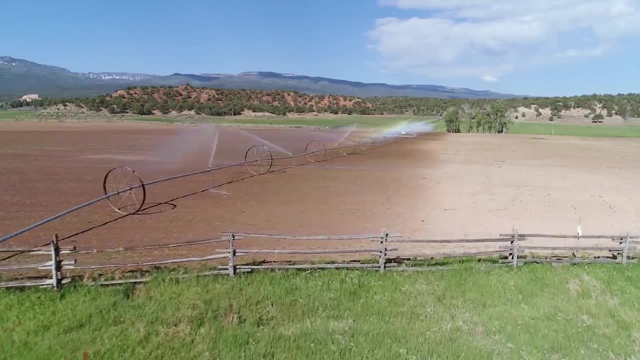 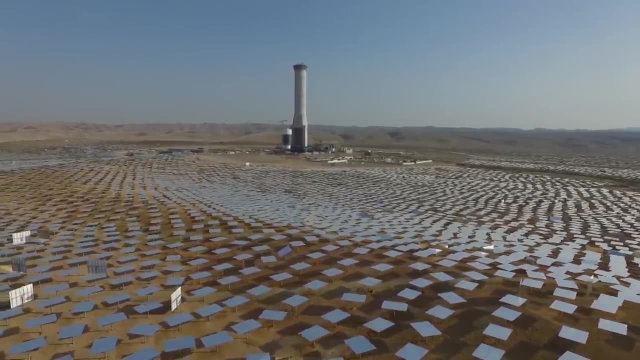 irrigate local farms to boost local economies even more. For this dream of turning the Earth's barren deserts into energy generation centres to come true, it has to be a grass roots movement, Not some new age imperialism megaproject. Not some new age imperialism megaproject. 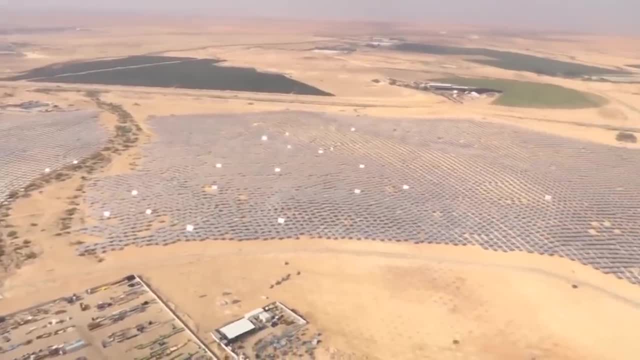 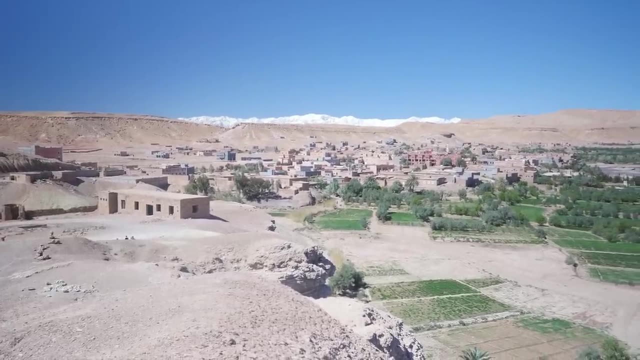 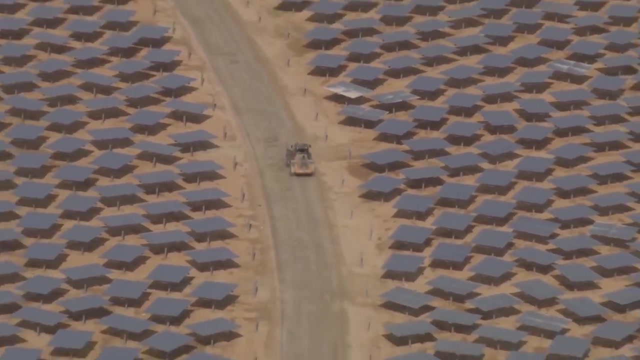 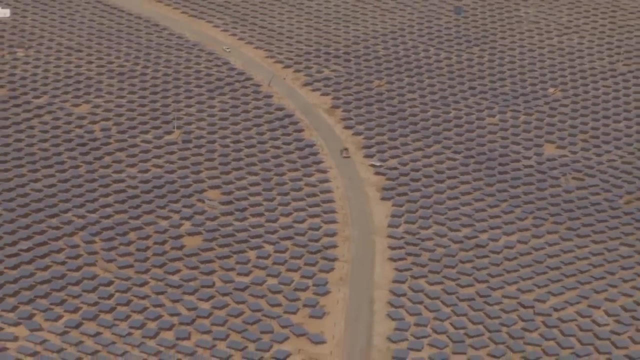 But is the eco-day21.. North Africa is one of the hardest hit regions in the world by climate change, with desertification and water scarcity becoming a serious issue. This plan, despite its surface level good intentions, sought to exploit countries that have suffered the most as a result of western industrialisation. 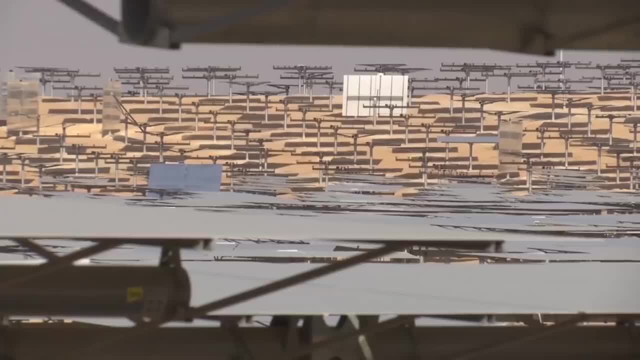 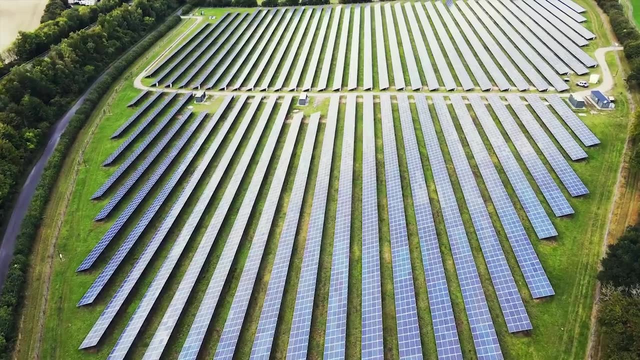 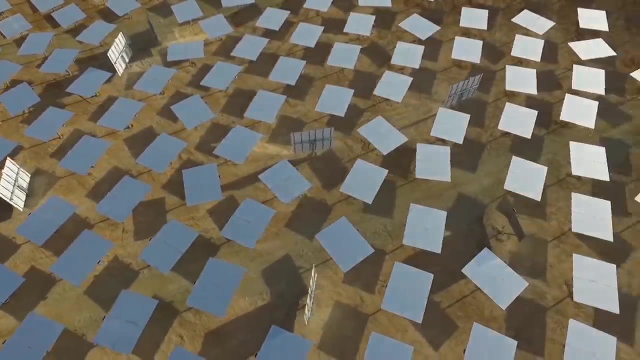 We don't need to look for the proof that this was their intention. They have theireurs. moment the technology developed to allow European countries to provide their renewable power needs within their own borders, the plan disintegrated. The plan was never about helping African nations. 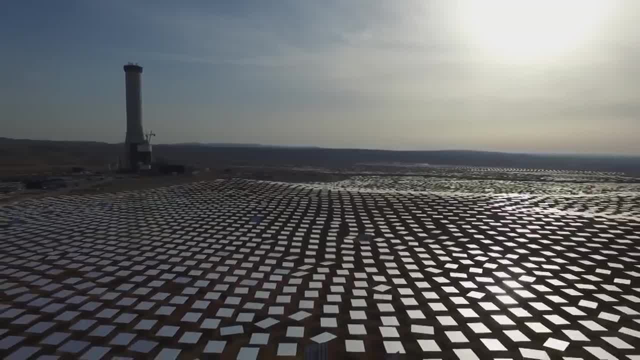 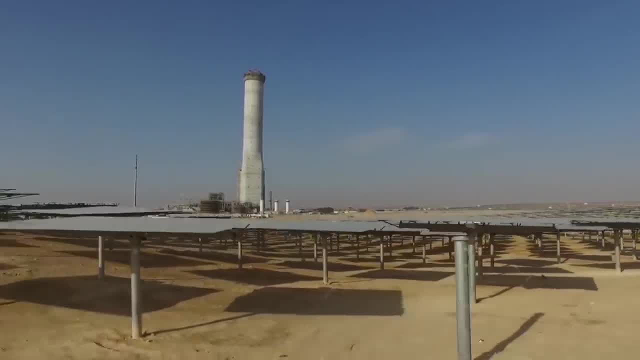 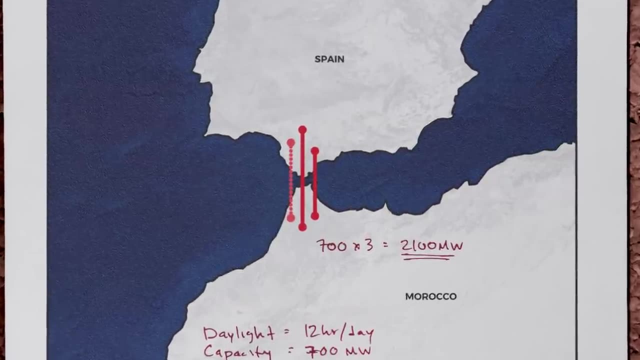 But the idea isn't dead in the water. These countries do have the natural resources to benefit from solar energy. Morocco is in the best position to lead by example. It's proximity to Spain allows relatively short interconnections to the European grid. It's government is. 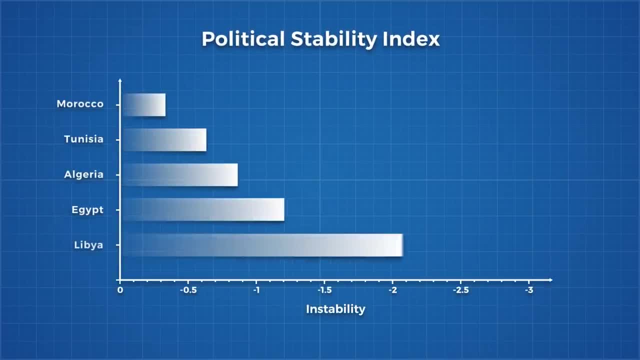 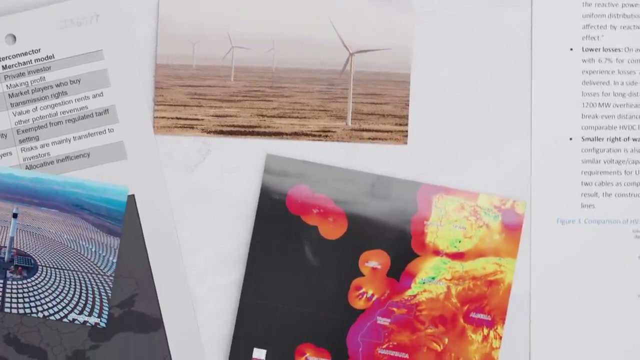 relatively stable compared to its North African neighbours, with a political stability index of minus 0.33.. Algeria, Tunisia, Libya and Egypt are all much lower, And while Morocco has abundant solar resources, it also benefits from consistent desert winds along its coasts. 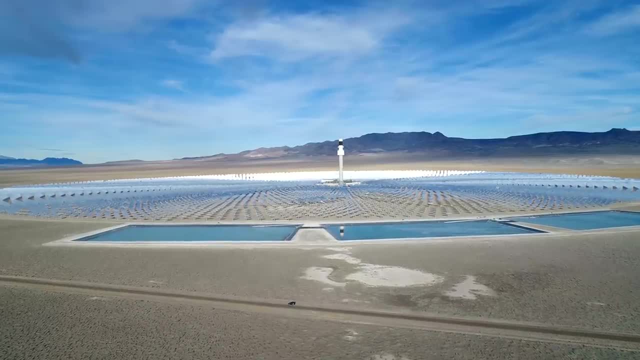 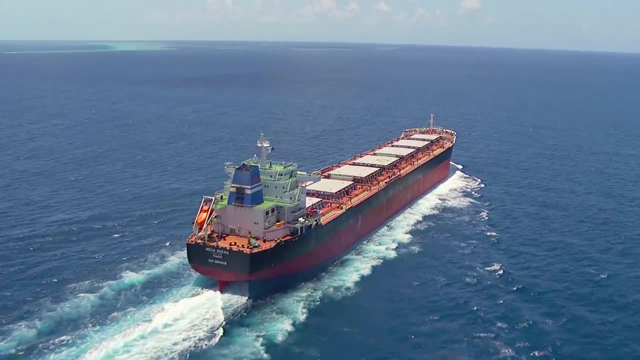 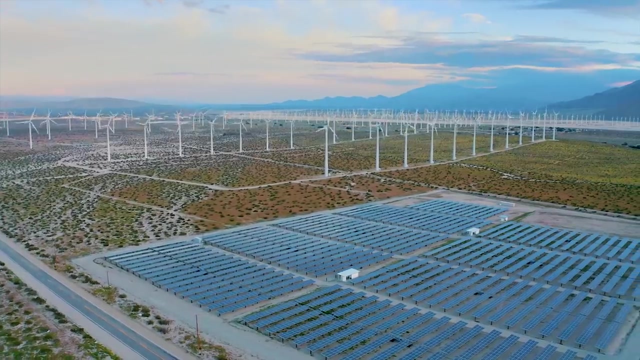 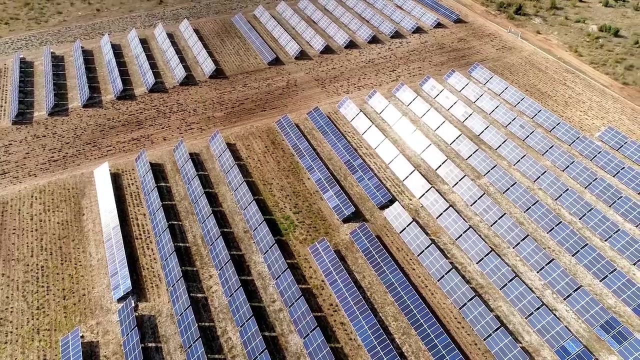 Morocco has the potential to invest in its own energy needs while exporting excess to Europe, Leading by example, Slowly shifting away from being a net energy importer of fossil fuels and becoming an energy exporter. Local infrastructure to benefit local people first. An African nation using its resources to benefit itself first and foremost. 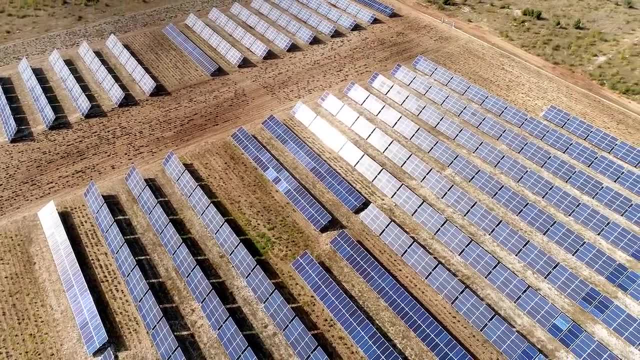 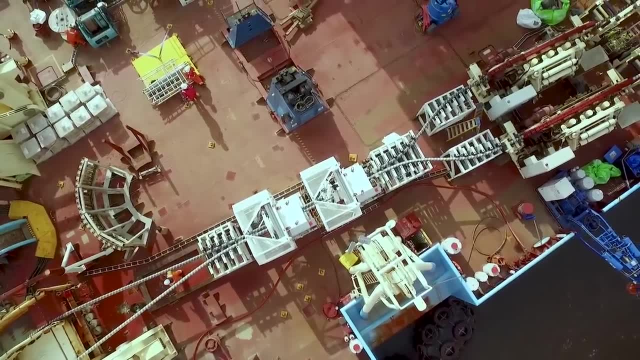 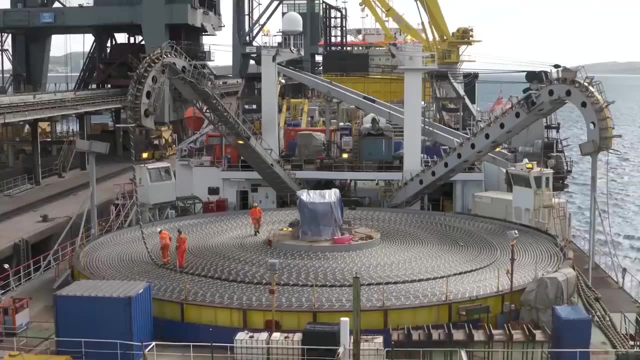 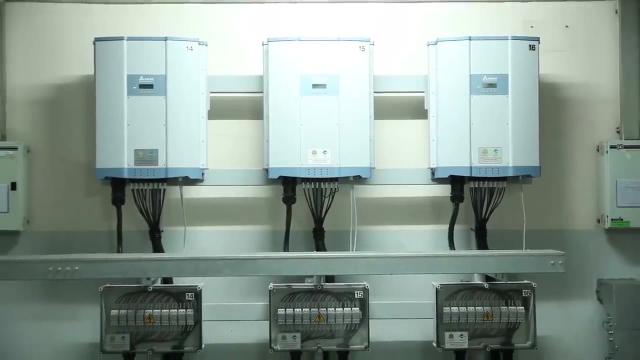 The potential for Africa's solar energy future is undeniable. The technologies to facilitate cross border energy trading exist and investments are happening to increase capacity for trade, with this third interconnector between Morocco and Spain funded equally by both sides, ensuring a level playing field, Figuring out the best practice for growing and improving. 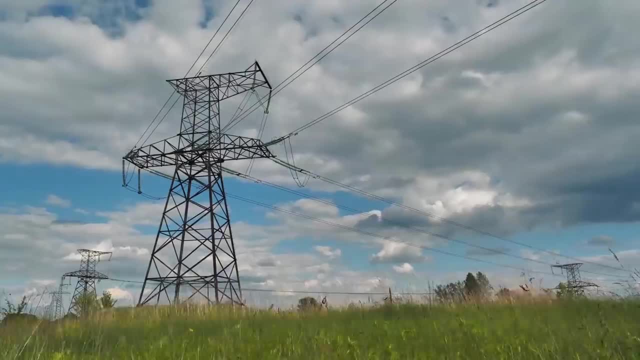 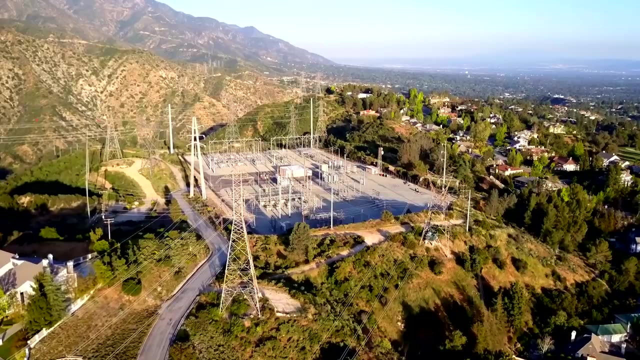 our electric grids is incredibly complicated. Electricity grids are effectively the largest machines on the planet. Hundreds of generators scattered across countries can be used to generate electricity and can be used to generate energy. Can be used to generate electricity and can be used to generate energy. Can be used to generate. 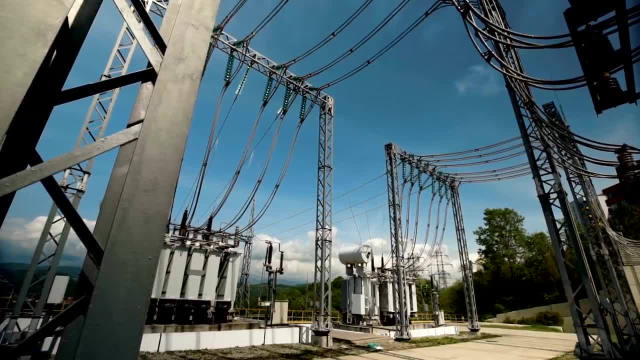 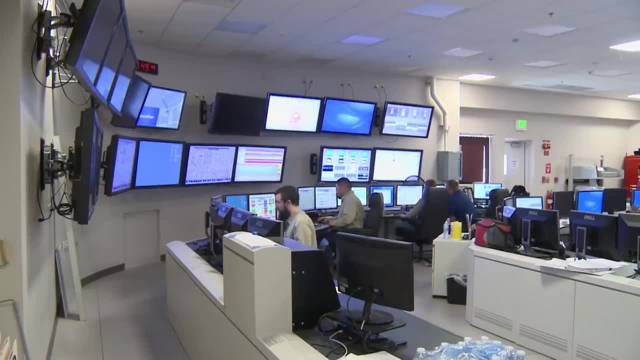 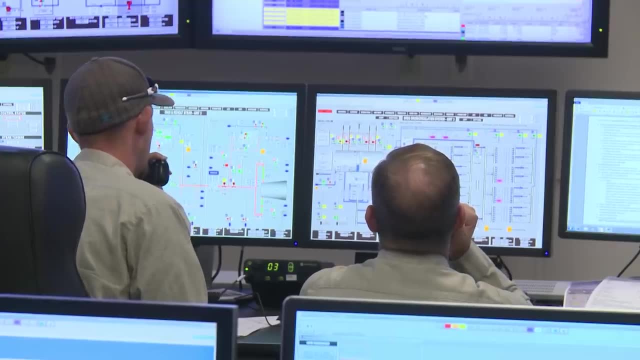 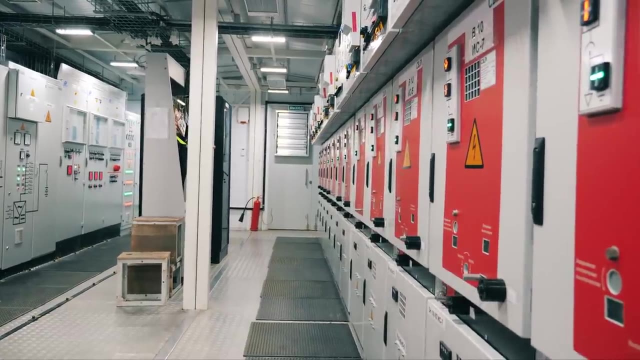 sensible decisions for a single human is impossible And more and more of the grid infrastructure is turning towards a smart grid controlled by algorithms. Battery farms employ coding and math experts to develop algorithms to allow them to buy and sell the electricity they store to maximise profit. And coding jobs like that are some of the best. pain and high. 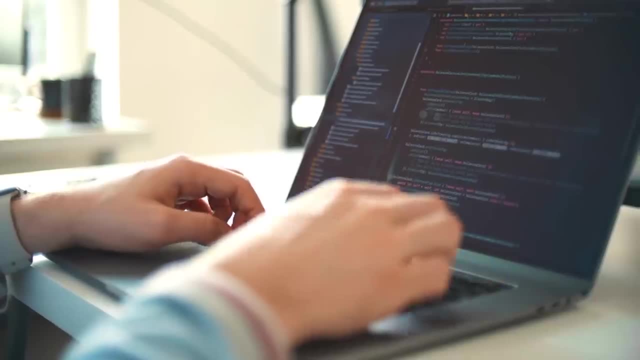 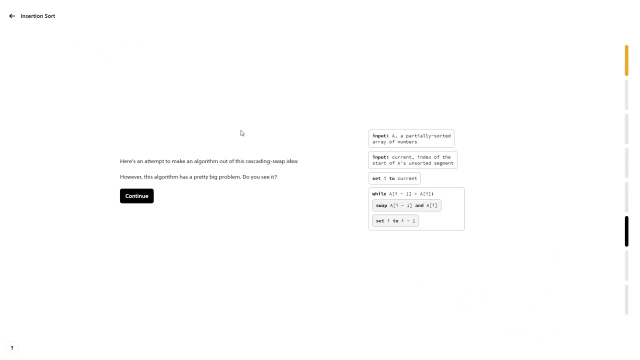 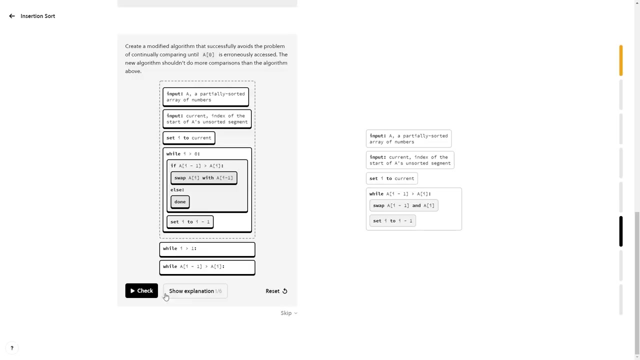 demand in the world today. Learning about algorithms and coding like this is an invaluable skill and, whether you are a high school student or experienced engineer, Brilliant is a great place to start learning and brushing up on your skills. I recently started the interactive course Algorithm Fundamentals and learned a ton of